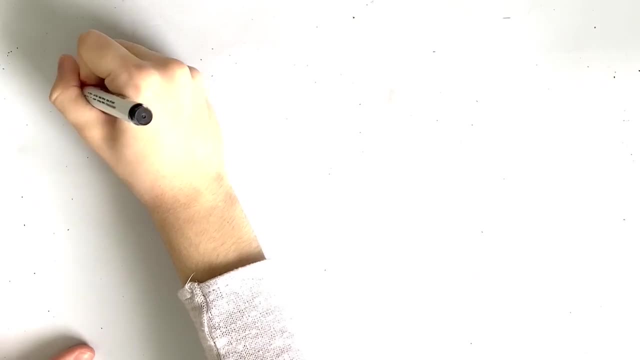 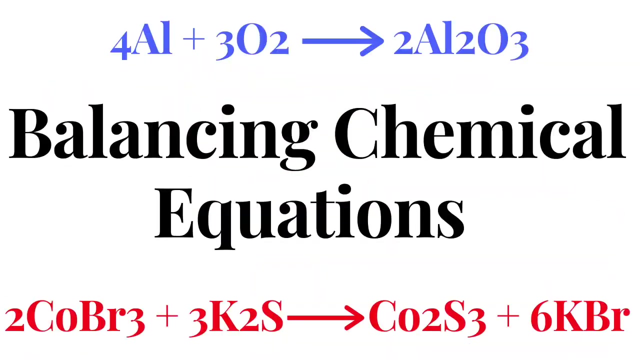 is sodium plus chlorine yields sodium chloride. If you are unsure as to how we balance the equation or why the elements have certain states, make sure to check out our other videos Balancing Chemical Equations and How to Figure Out the States of an Element or Compound. Secondly, a multivalent metal reacts with a non-metal to form various ionic compounds. For example, copper plus chlorine yields copper chloride and copper plus chlorine yields copper chloride. This is because copper, as we mentioned, is multivalent. Copper has a charge. 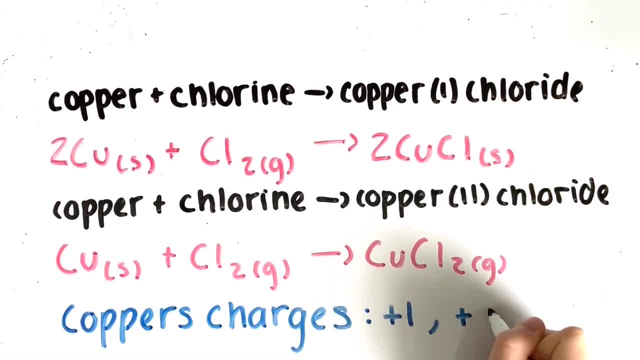 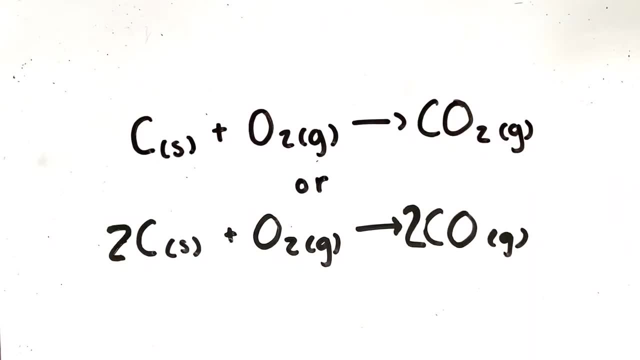 of positive one and positive two, therefore yielding two different results. Thirdly, two non-metals combine to form a molecular compound. For example, carbon plus oxygen yields carbon dioxide and carbon plus oxygen yields carbon monoxide. They are both non-metals and carbon is multivalent, so they form molecular compounds. 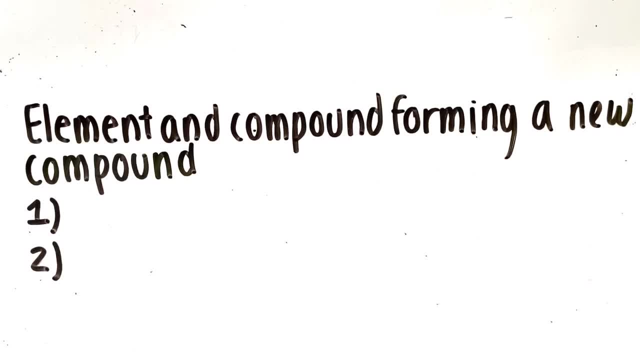 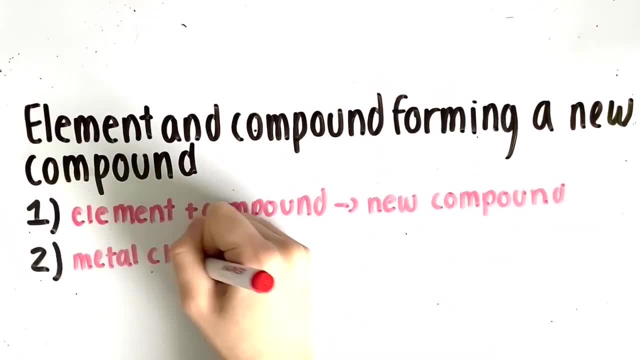 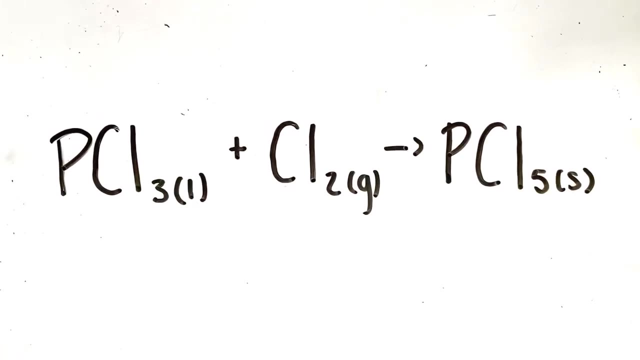 Next, an element and compound forming a new compound. There are two different ways that it can occur. Any element and any compound forming a new compound and a metal chloride plus oxygen gas yields a metal chloride. An example of an element and a compound forming a new compound is phosphorus trichloride plus chlorine gas. 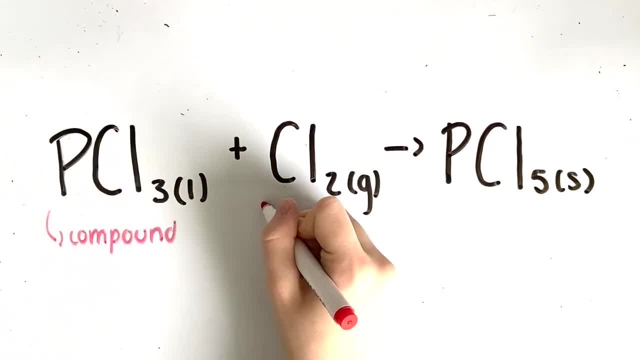 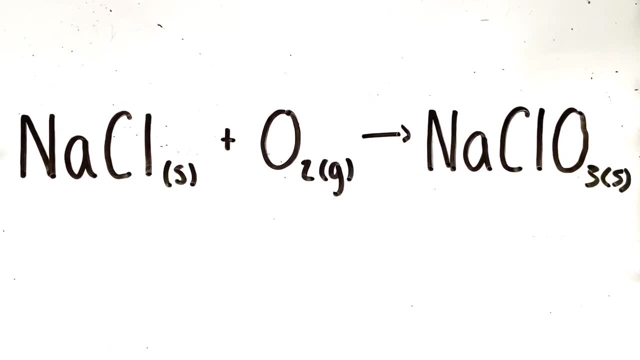 yields phosphorus pentachloride. Phosphorus trichloride is our compound and chlorine gas is our element, and phosphorus pentachloride is our new compound. An example of a metal: chloride plus oxygen yields a metal: chlorate is sodium. chloride plus oxygen gas yields sodium. 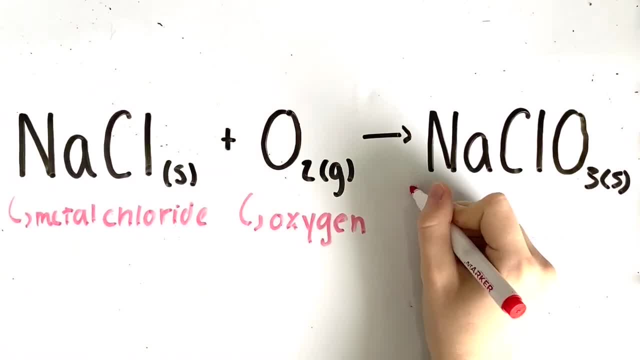 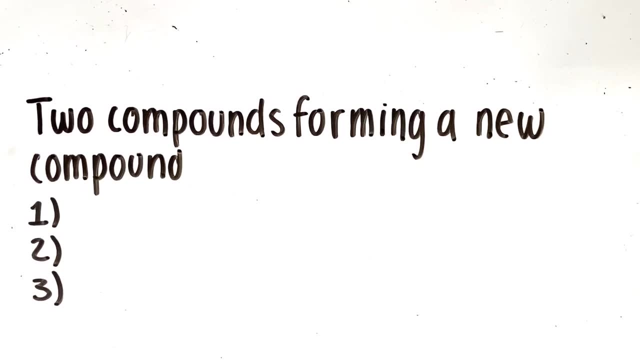 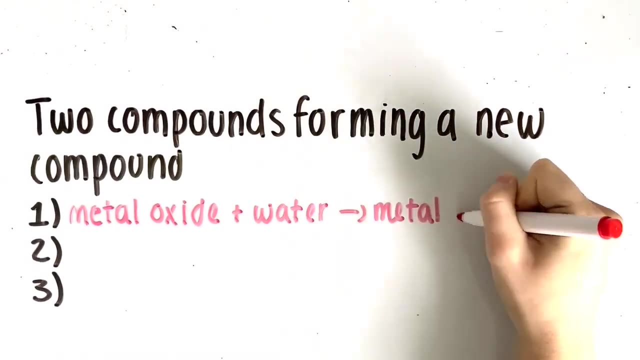 chlorate. Sodium chloride is our metal chloride and oxygen gas is oxygen and sodium chloride is our metal chlorate. Finally, two compounds forming a new compound. There are three different ways that two compounds can form a new compound: A metal oxide plus water yields a metal hydroxide. A nonmetal oxide plus 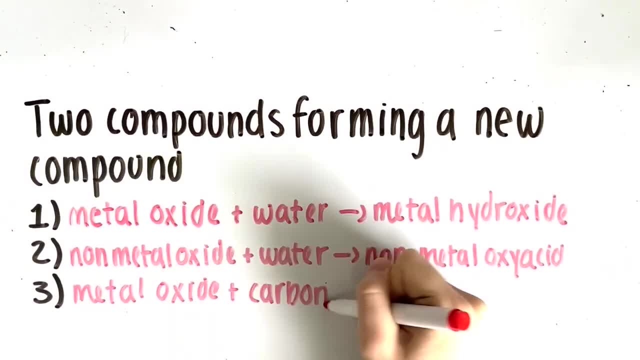 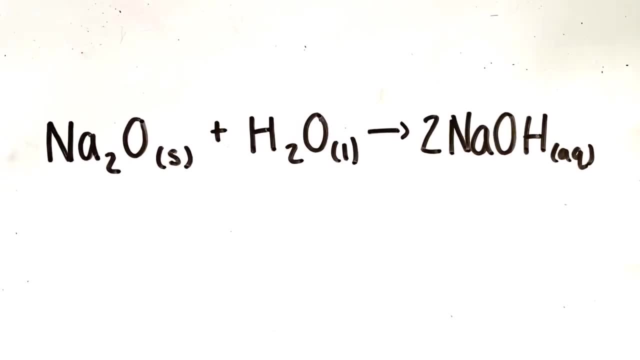 water yields a nonmetal oxy acid, and a metal oxide plus carbon dioxide yields a metal carbonate. Firstly, a metal oxide plus water yields a metal hydroxide. for example, sodium oxide plus water yields sodium hydroxide, The, The metal oxide, is sodium oxide and H2O is the water, and it yields sodium hydroxide, which 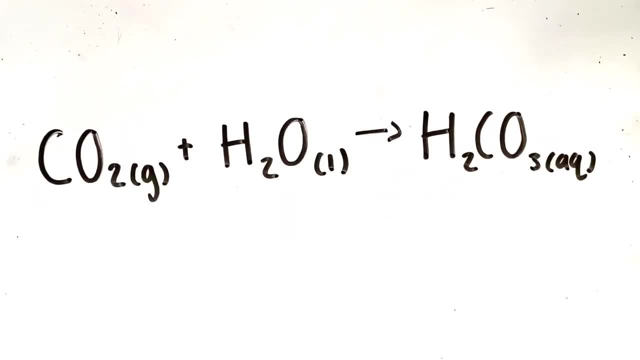 is the metal hydroxide. Secondly, a non-metal oxide plus water yields a non-metal oxy acid. For example, carbon dioxide plus water yields carbonic acid. Carbon dioxide is our non-metal oxide and H2O is water and it yields carbonic acid, which